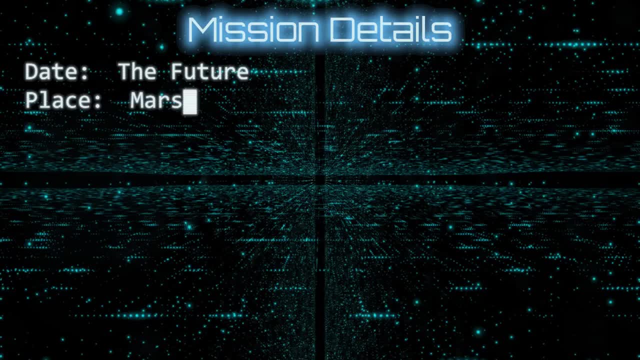 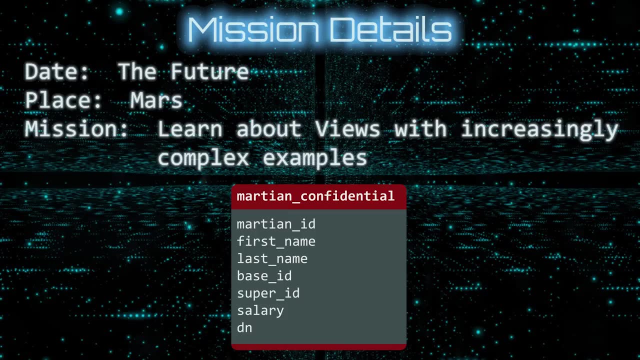 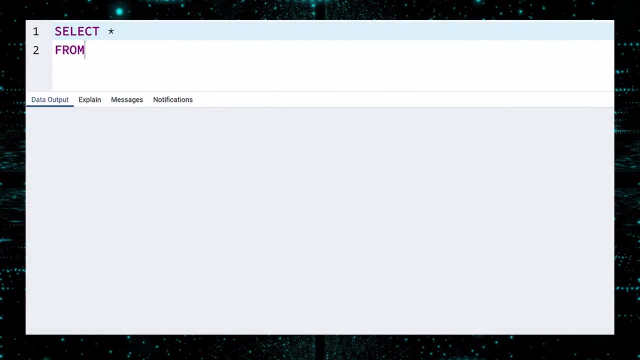 in the future, The place Mars, The mission: learn about views. To start, suppose we have a table called Martian Confidential. This table contains information on every person who is living on the planet. Let's take a look at the data in the Martian Confidential table. 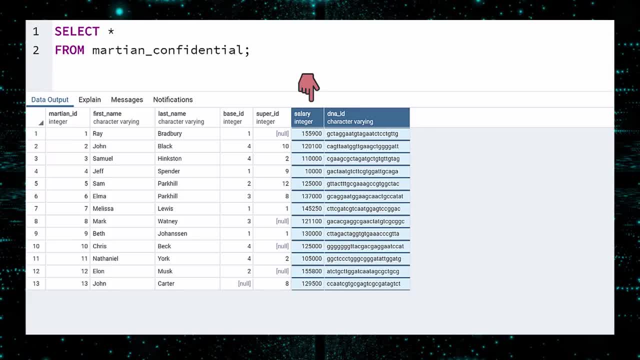 Two of its columns contain sensitive information. The salary and solar credits should not be available to everyone, And the DNA ID is extremely sensitive. Unauthorized cloning is a growing problem in the remote colonies. How do we give engineers access to some of this data? 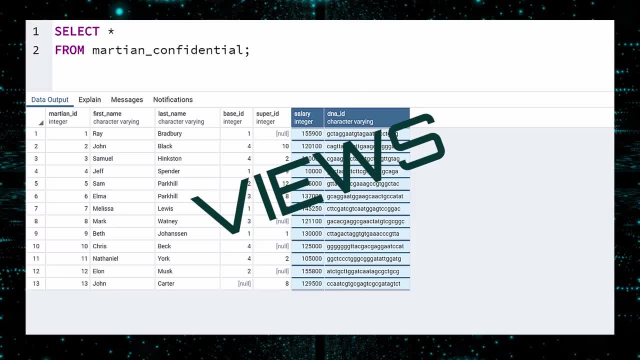 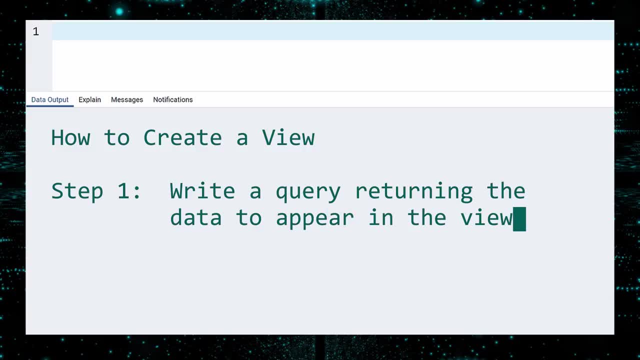 but not these two columns, By creating a view. The first step in making a view is to write a query returning precisely the rows and columns you want in your view. We have been instructed that it is okay to share all data except the salary and DNA ID columns. 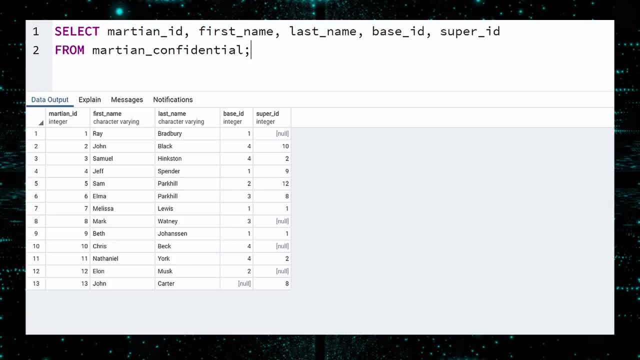 Execute To create a view from this data. insert a line above the query Write create view and give your view a name. We will call this view Martian Public. Then write as. That's all there is to it. Run this query, The view is created. You can now treat Martian Public as a table. 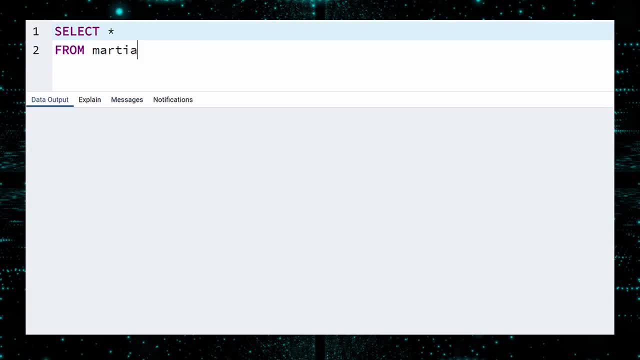 A quick select shows that the confidential data is not present. And look what happens if you try to select the confidential data, You would never know it was there. That data is now a rumor, recognizable only as deja vu and dismissed just as quickly. This is an important benefit of views. 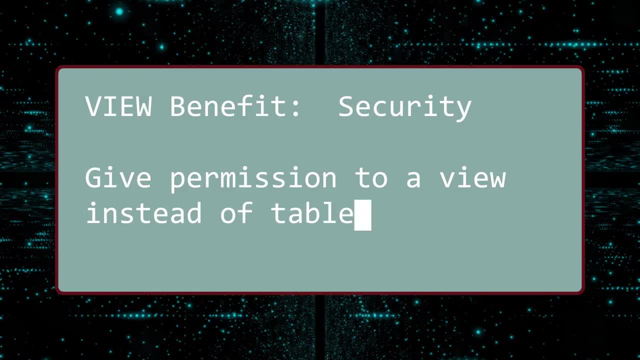 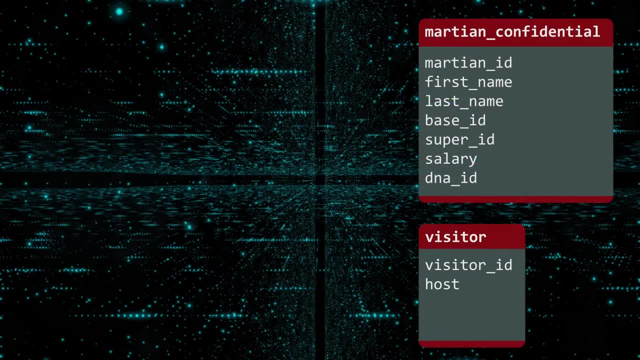 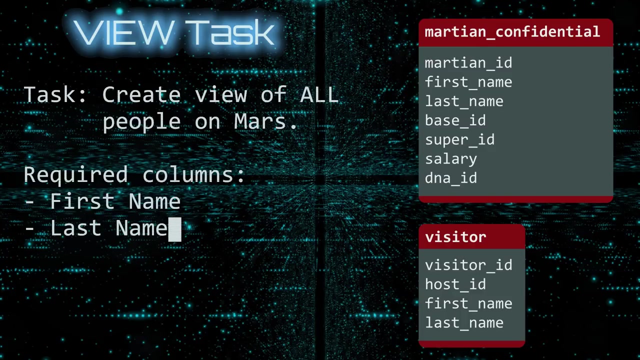 Security. By giving engineers access to views instead of all the underlying tables, you control the data they can see. Let us introduce another table to our database: Visitor. This table holds a list of all people currently visiting Mars. Here is our task: Create a view that contains a list of all people on Mars. This view should contain their first name, last name, a unique ID and their status: Martian or Visitor. 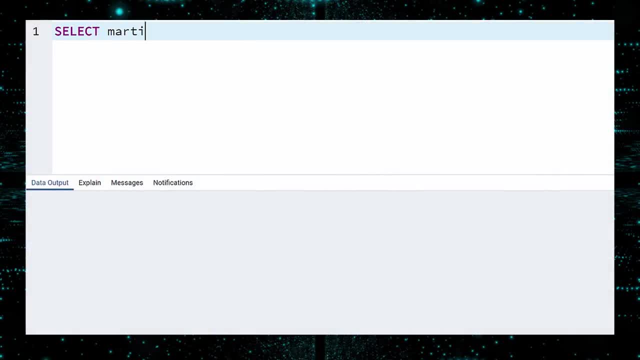 We start by writing the query to generate this list. Our first select gives us the information we need from the Martian table. Each person in this table IS a Martian, So in the select clause include a Marsian String and call the column containing this String Status. 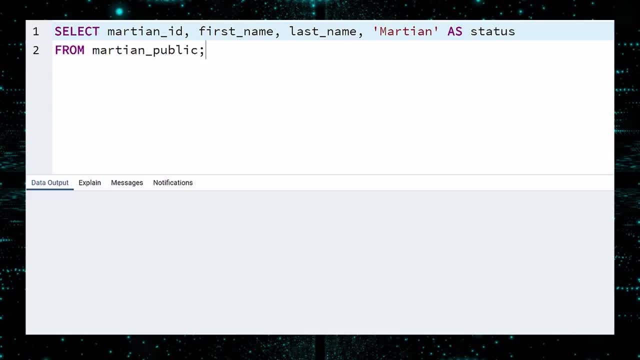 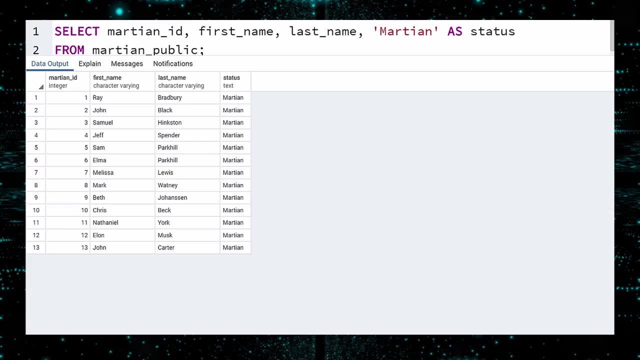 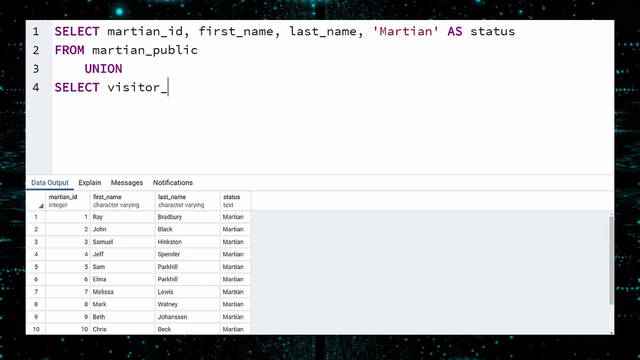 Execute. This gets us part way there. We also want the names, status and IDs of the visitors too. One way to combine two queries is with the Union Command. This will combine the results of 2 select woman names. You only need to be sure to line up columns of the same type. acceptau questions of the same type. 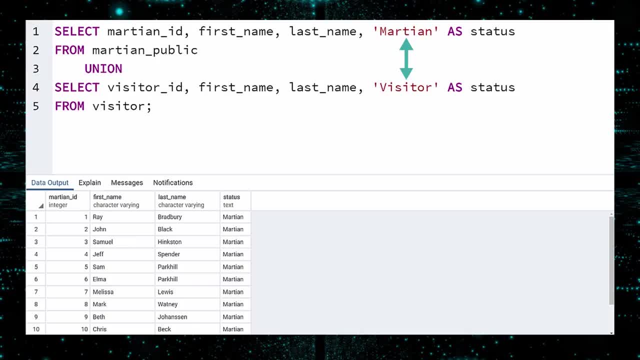 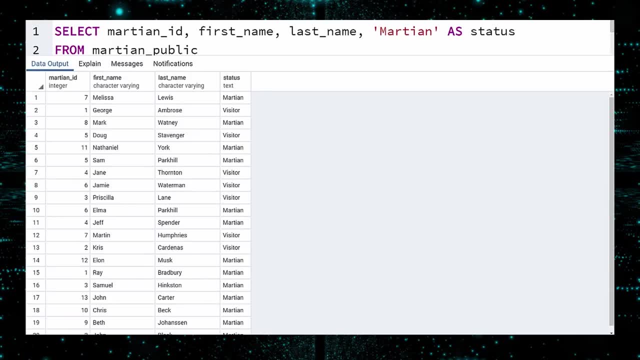 in your two select queries. The two selects need to have the same number of columns and the types must be the same Execute. We are closer, but one problem remains: the ID. Some visitors and Martians have the same numeric ID. 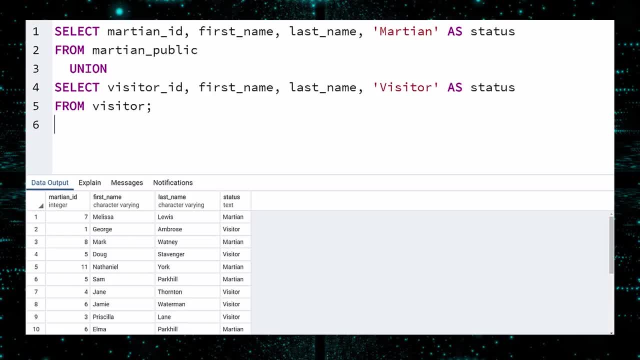 One solution is to preface each Martian ID with a letter M and call this column simply ID. We do this using the CONCAT function And in the VISITOR SELECT query we will put a V in front of each ID. Now execute once more. 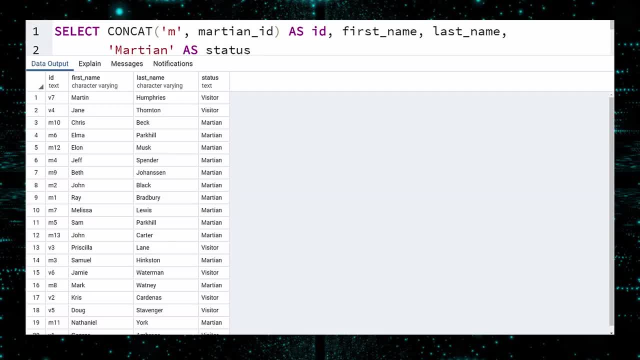 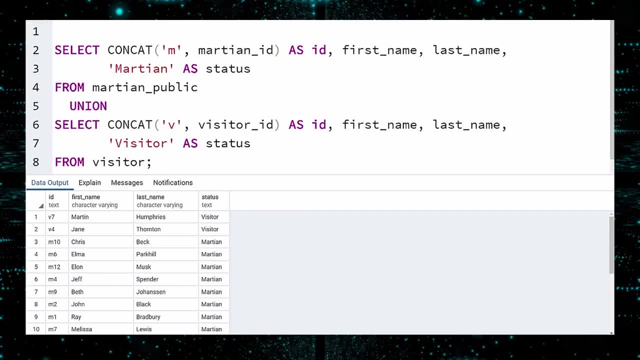 We now have a list of all people on the red planet: their names, status and a unique ID. We can now turn this into a view. At the top, insert CREATE VIEW with the view name. We will call this People on Mars. 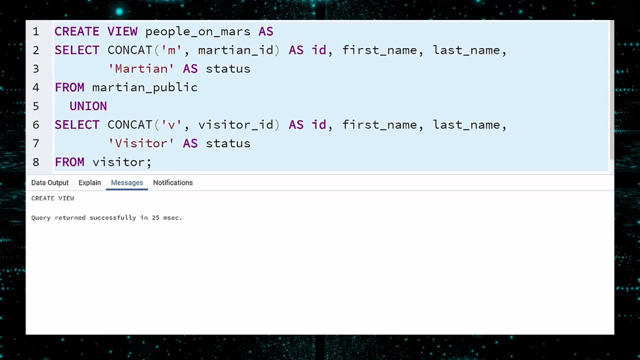 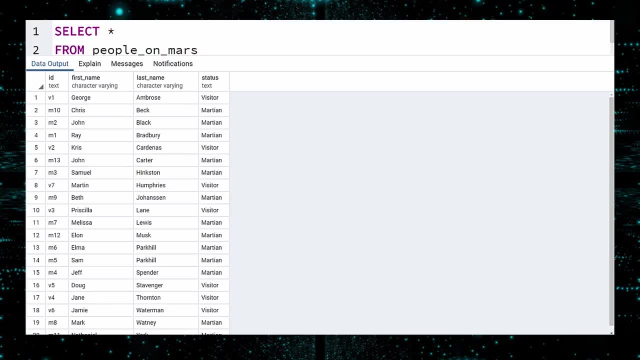 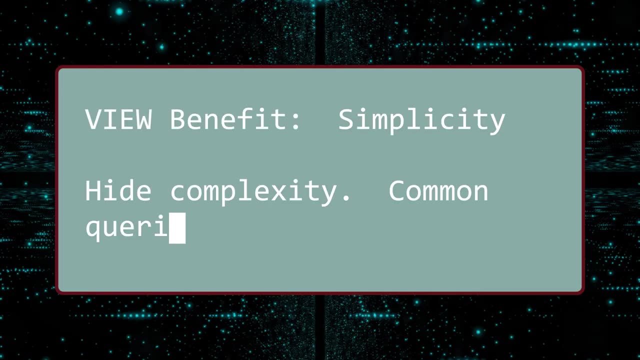 end it with an as and execute. Engineers can now easily query the list of people on Mars by using this view Execute. This is another benefit of views simplicity, Instead of requiring people to query two tables or know how to use Union. 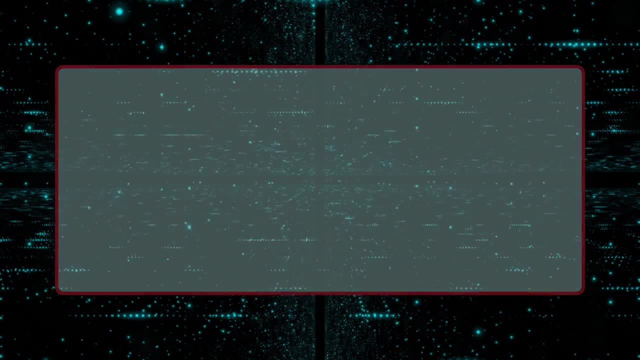 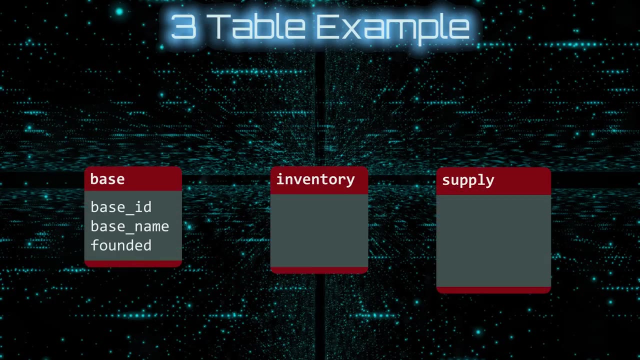 they can simply write a SELECT using this view. For our next example, we will use three tables in the Martian database: Base, Inventory and Supply. The Base table holds information on all the different habitats on Mars. The Supply table lists all items available. 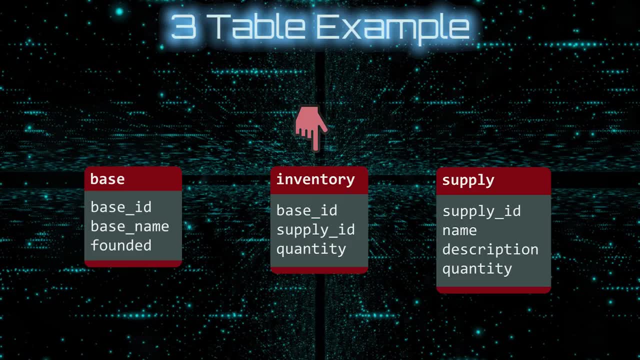 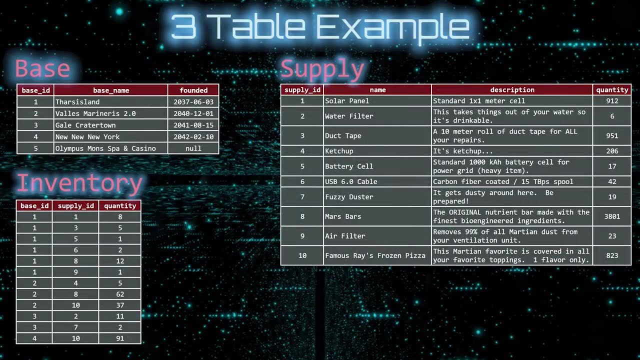 in the Central Martian Distribution Center And the Inventory shows what supply items are available at each base and in what quantity. Here are the data for the three tables. Look closely at the Inventory data. If a base does not have a supply item in stock. 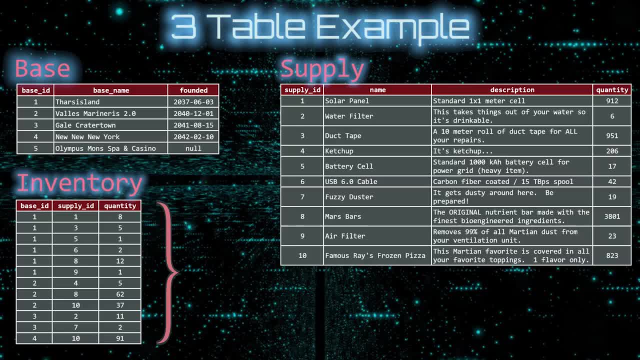 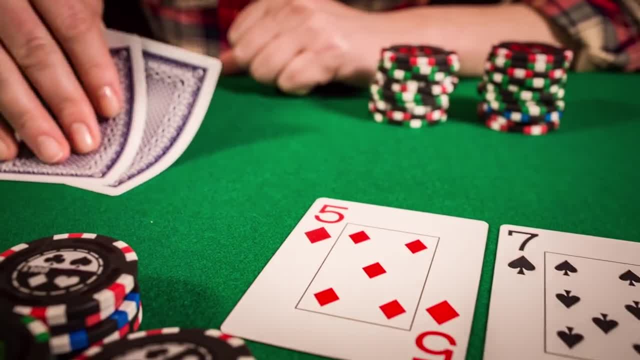 it is not listed with a quantity of zero. Instead, it is not in the table at all. One might debate this design choice. Regardless, we have to play the cards we are dealt, especially if we want to be ready when the Olympus Mons Spa and Casino opens later this Sol. 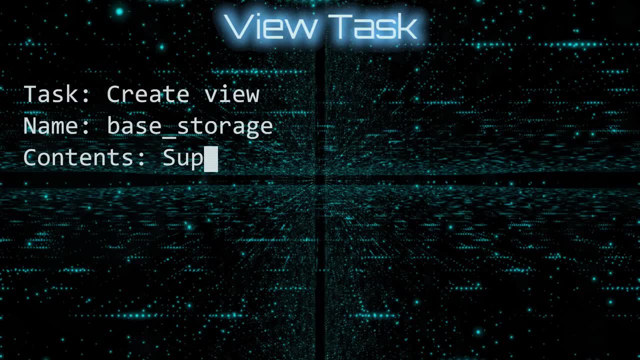 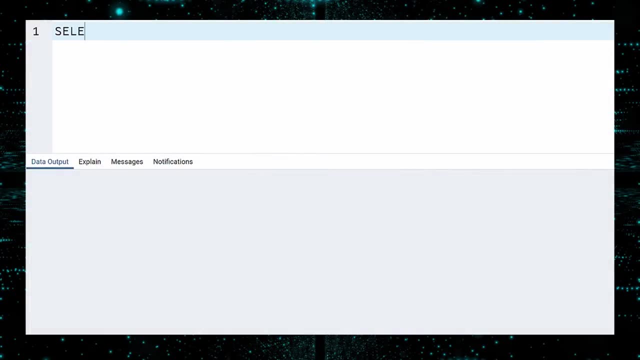 Our task is to create a view called Base Storage, showing the quantity of all supply items in stock at each base. As a first step towards building the query, select the Base ID, Supply ID and Supply Name for all possible combinations of Base and Supply item. 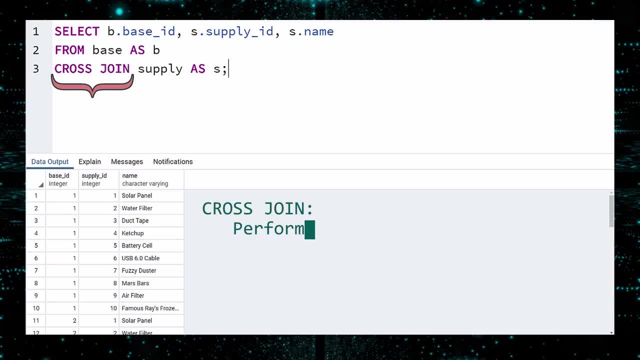 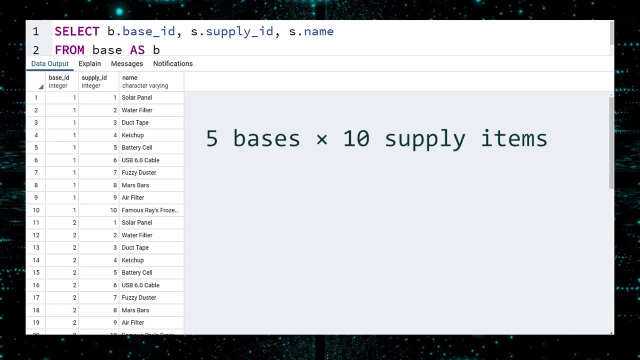 This is done with a cross join. This type of join performs a cross product between the two tables, That is, it connects each row from the first table with each row in the second table. This gives us all possible Base Supply combinations, Since there are five bases and 10 supply items. 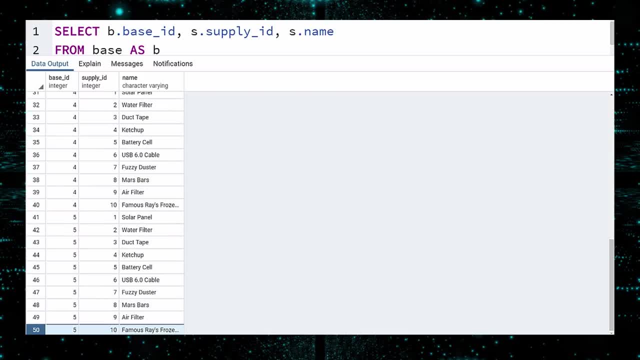 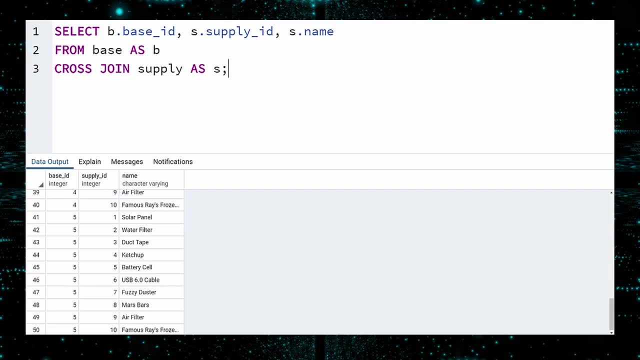 there should be 50 rows in this cross join And there are. What remains is the quantity of each supply available at a given base. We can obtain this value from the inventory In the SELECT clause. embed a SELECT to get the quantity from the inventory. 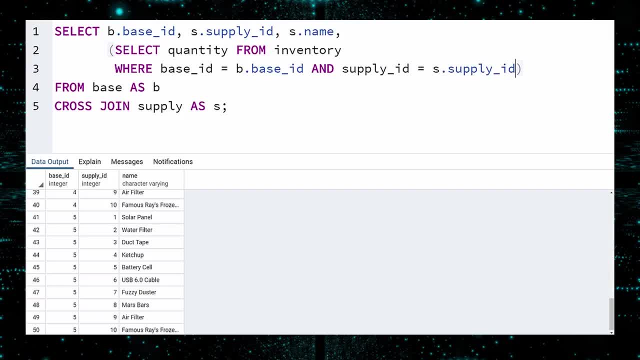 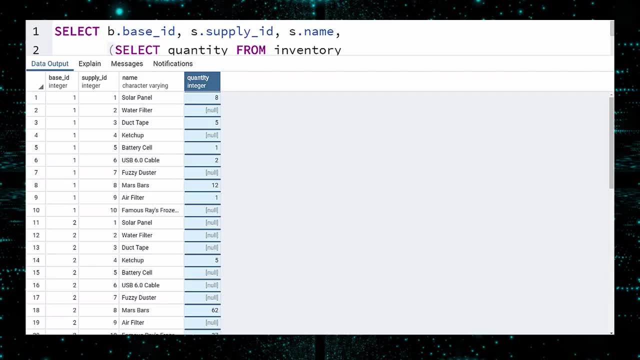 for this row's Base ID and Supply ID Execute. Unfortunately, some of the values are null. We do not want engineers to be concerned about nulls, so we will replace all nulls with zero. We can do this with the COALESCE function. 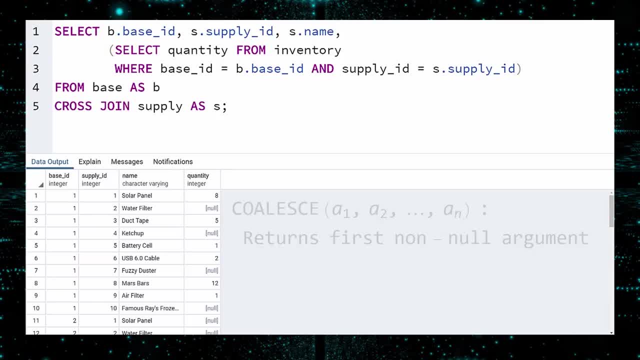 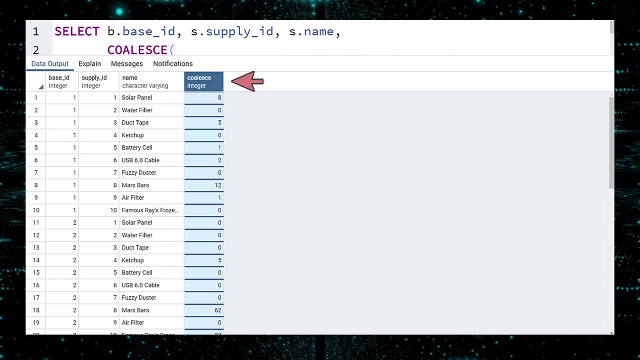 This function returns the first non-null value it encounters. If the inventory table does not contain the quantity, it returns null. In this case, the quantity is actually zero. Execute Rumble. The column name is called COALESCE, not a terribly descriptive name. 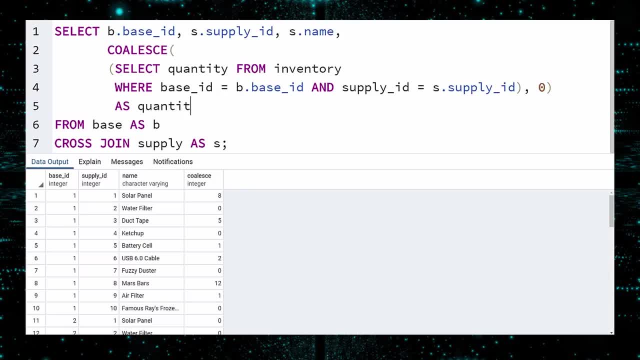 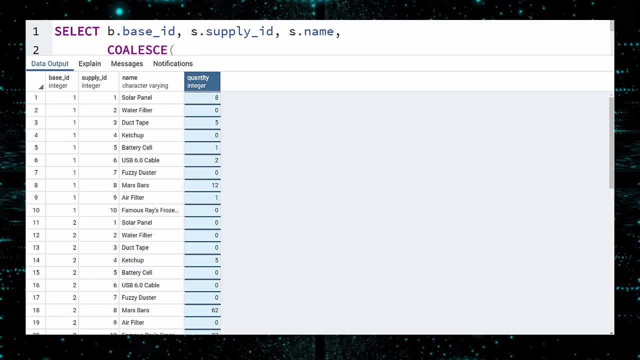 So we alias the output of the COALESCE function as quantity Double execute. Now we are talking. This is the query we are looking for. All that remains is to turn this into a view, Return to the top and write the CREATE VIEW clause. 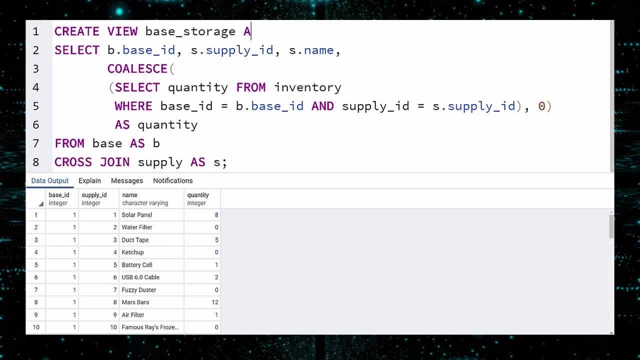 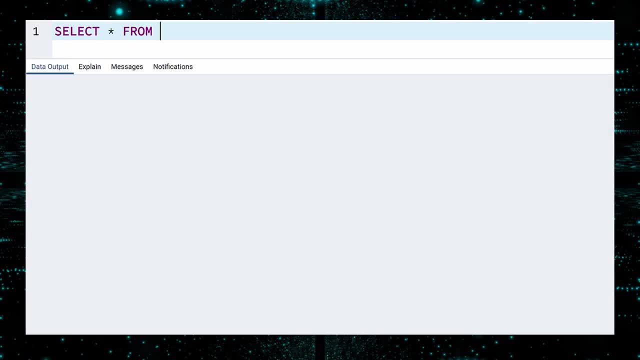 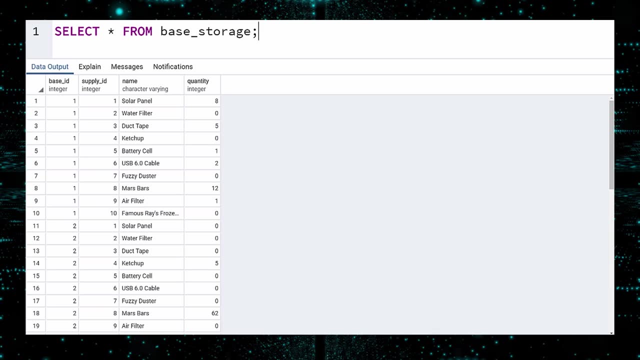 As in start, end and end. As instructed, we will call this view Base Storage Run Success. Let us now admire this view, And what a wonderful view this is. Our users can now query this view while the database designers continue to debate.